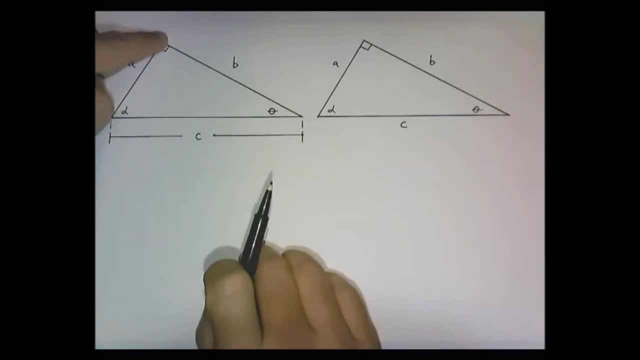 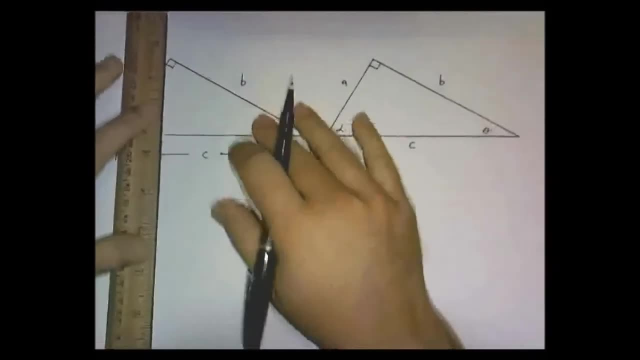 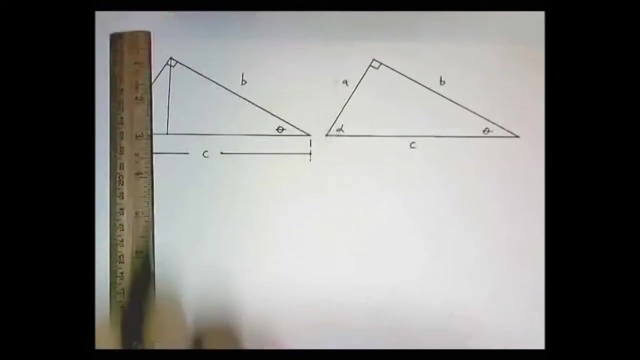 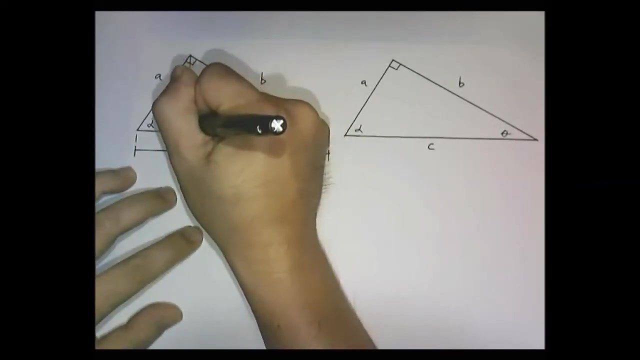 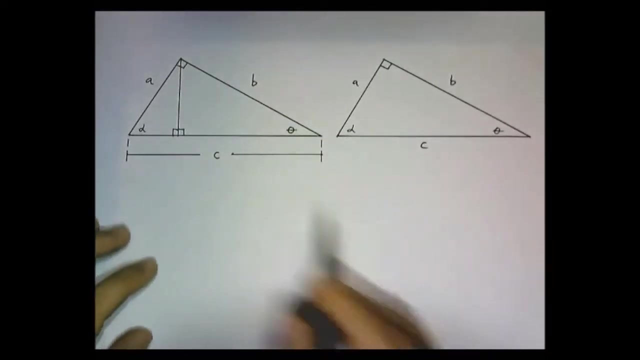 a line straight down from here to here, and then this line I inscribe is going to be a right angle to this line. Let me go ahead and do that. This line is at right angles to this surface, so that's a right angle there, and then this is a right angle here: The distance. 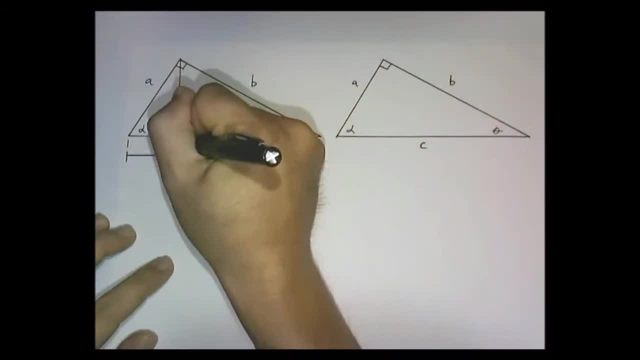 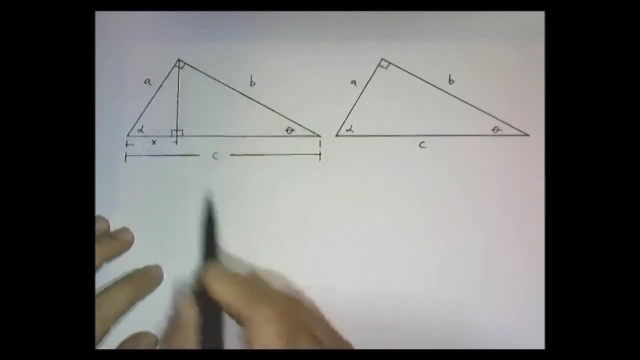 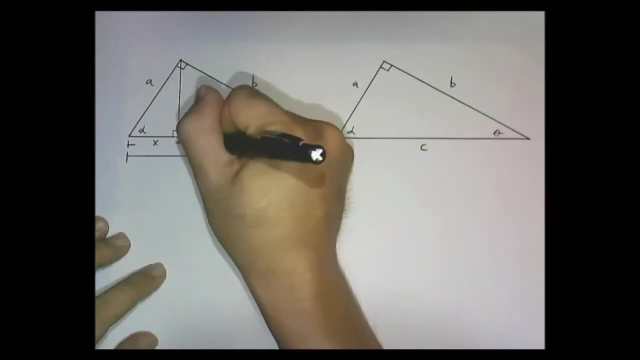 from here to here. I'm going to call x. Now, if the length of this entire side is c, then this distance here is c minus x, So x, c. this is c minus x, So I'm going to write that in. 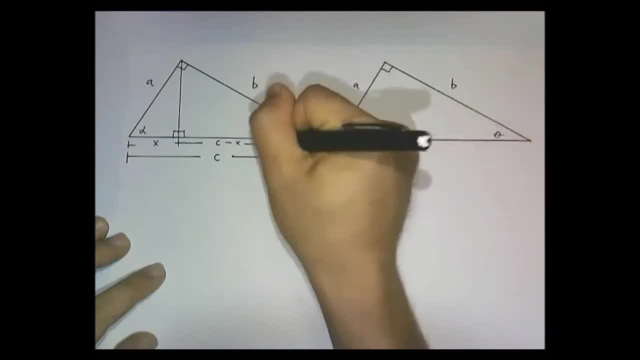 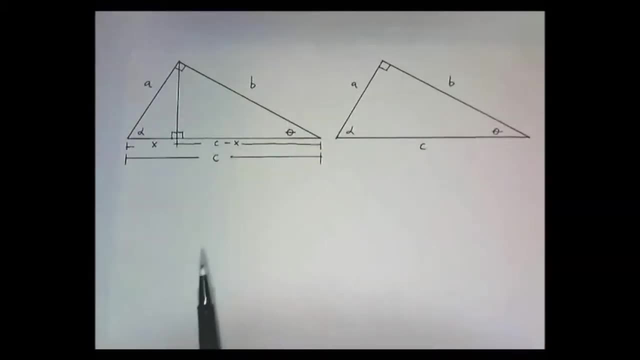 C minus x. Alright, we'll do that. Alright. now the idea of similar triangles is that if two triangles share two identical angles, then their third angle has to be the same. So, for example, this smaller triangle right here has the angles alpha and the 90 degree angle, And then this triangle right. 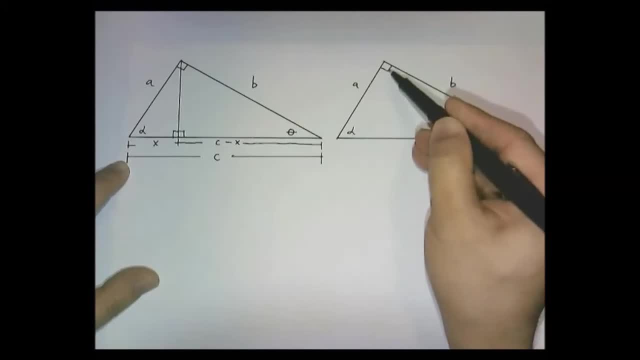 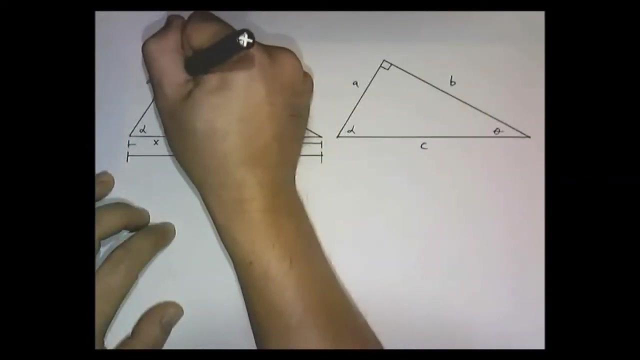 here has the angle alpha and a 90 degree angle and an angle theta. Well, that means that since alpha and a 90 degree angle are shared between these two triangles, that means this angle here has to be theta. So I'm going to inscribe that right here. If you take a look at this, 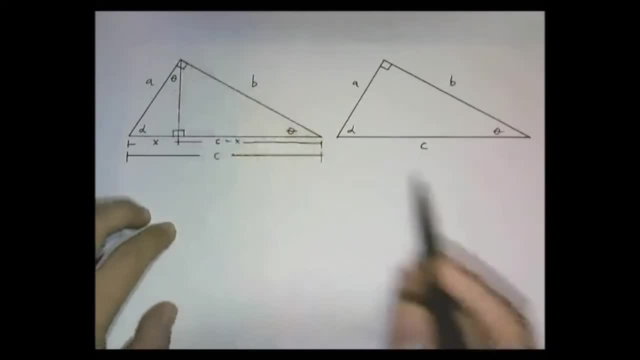 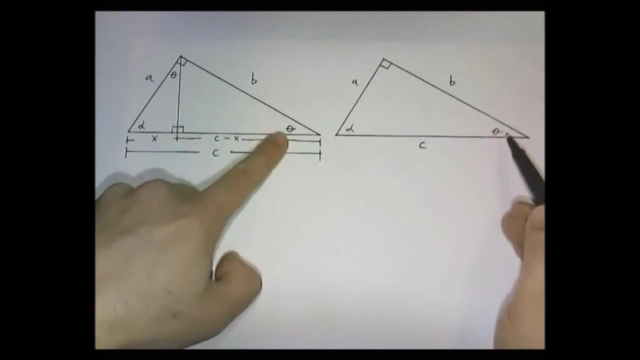 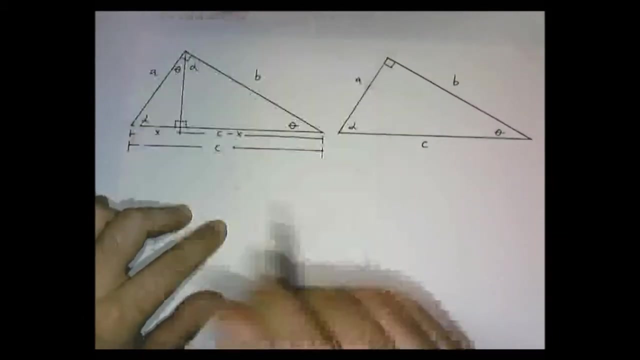 other, slightly larger triangle right here. it has the angle 90 degrees, just like this one, and it has the angle theta, just like this one. Well, if these two triangles share the angles 90 degrees and theta, and if this angle is alpha, then this angle up here has to be alpha. 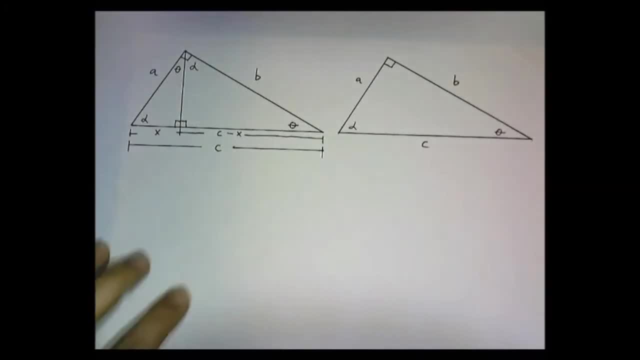 Alright, now what I'm going to do to differentiate the three different triangles, we see one, two and three. the big triangle I'm going to sort of color things in. So the small triangle I'm going to color in with the color pink. So let's just fill this up with some pink. 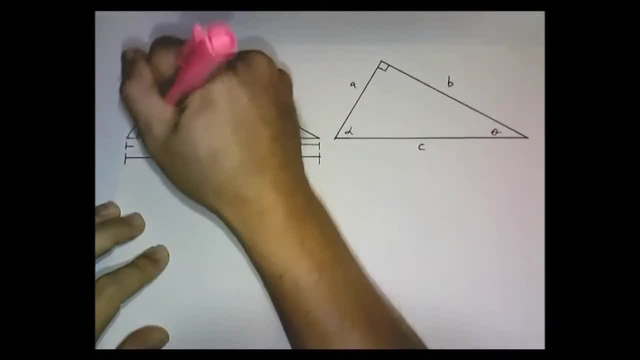 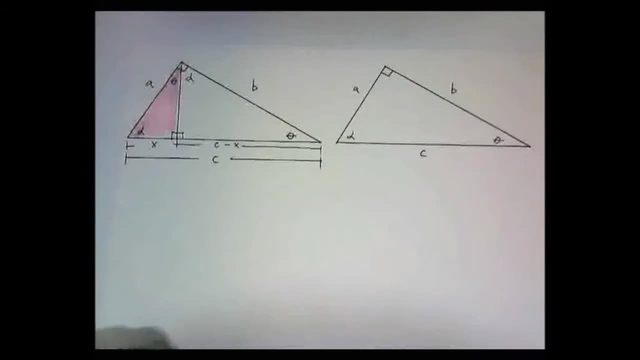 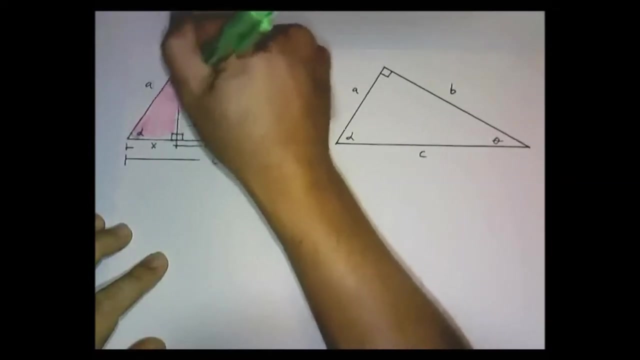 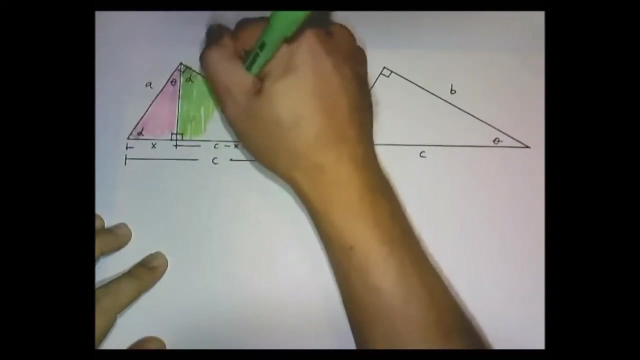 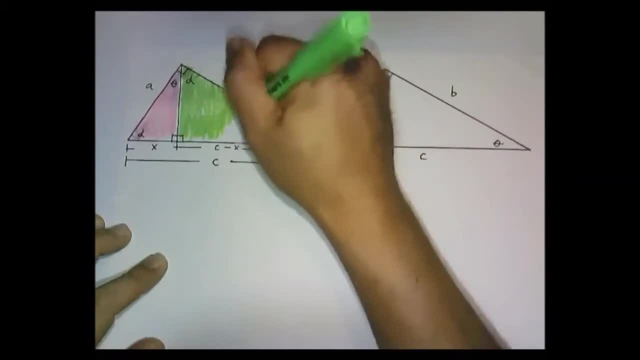 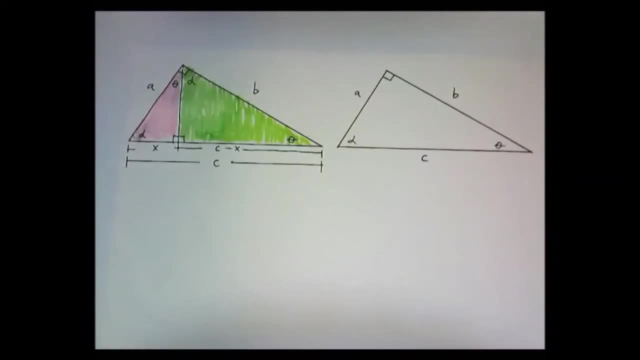 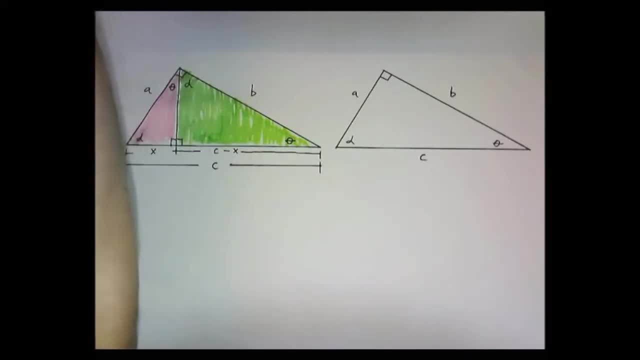 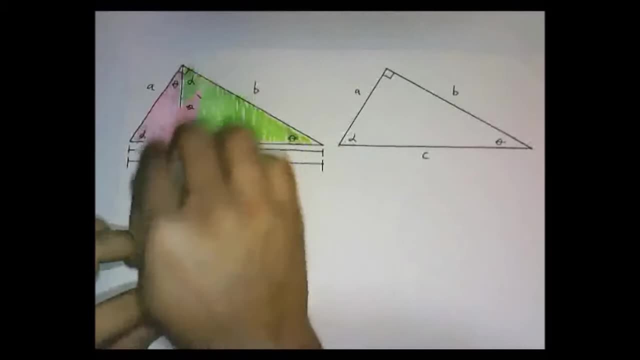 All right. so what I'm going to do now is I'm going to sort of place some cutouts on top of the triangle. So this pink triangle- right, pink triangle, right here I'm going to put a pink triangle on top to represent it, And 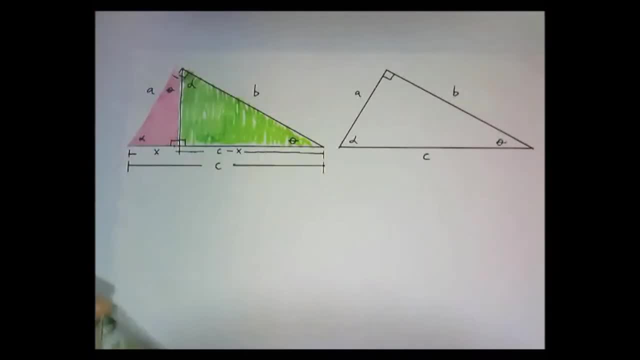 then this green triangle here. I'll put a green triangle here to represent it. All right, Now what I'm going to do is I'm going to take these triangles and flip them over and move them to a different location. So I'm just going to take this one and I'm going to move. 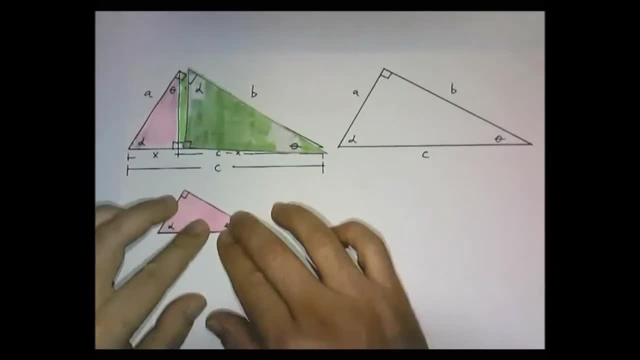 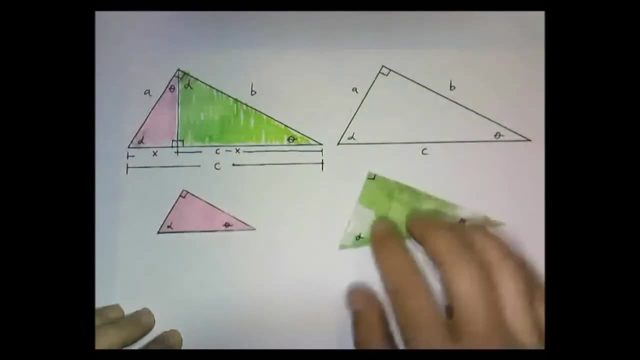 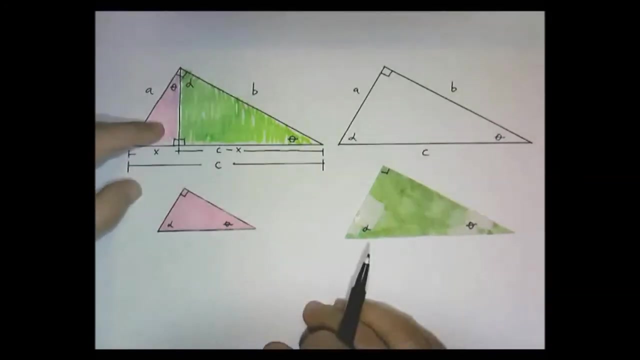 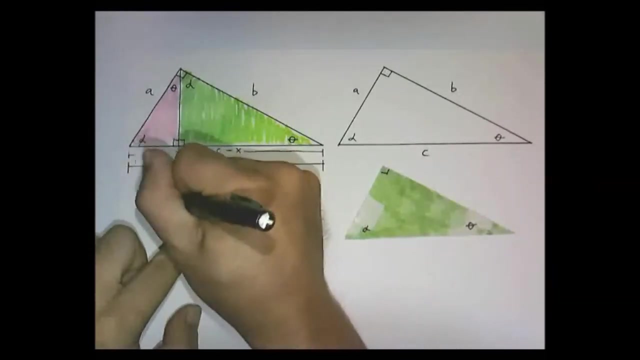 it down here like that, And then I'm going to take this one and move it over here. Just flip it and move it over. All right Now. this pink triangle is this pink triangle. This side x on this pink triangle is x right here. So this side x corresponds with that side. 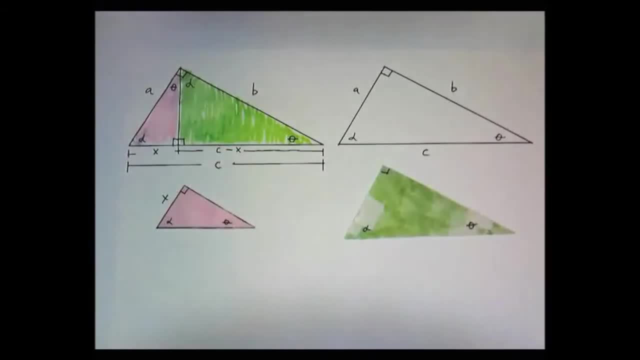 x, They're the same. And then what else do we have? This side a, the hypotenuse of the pink triangle, the side opposite the 90-degree angle, that's this side right here. So a, and then side a, right. 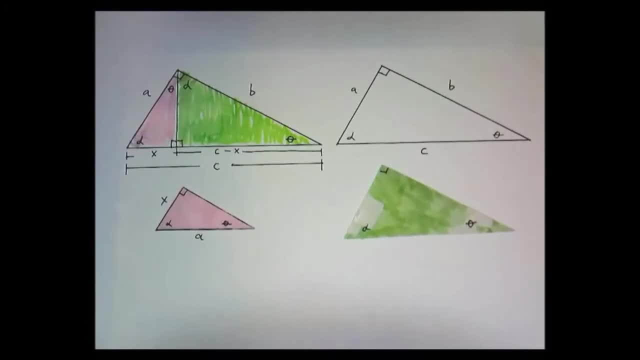 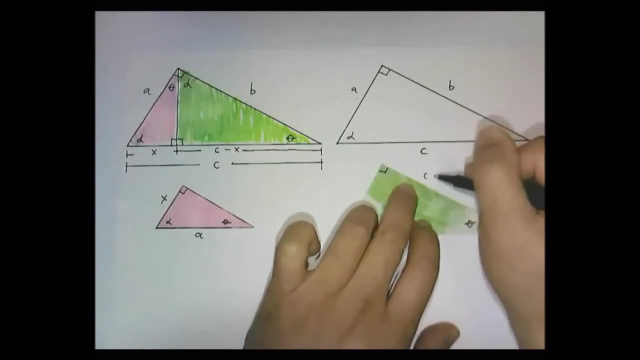 there. I'm going to do the same thing with the green triangle. Let's see here This side. here: c minus x. that corresponds with this side right here. Okay, So this is c minus x. right there, C minus x is opposite. 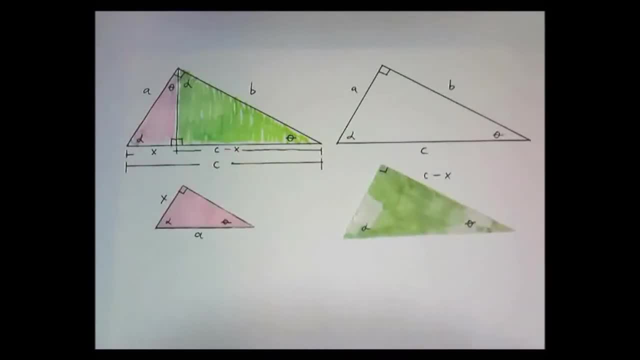 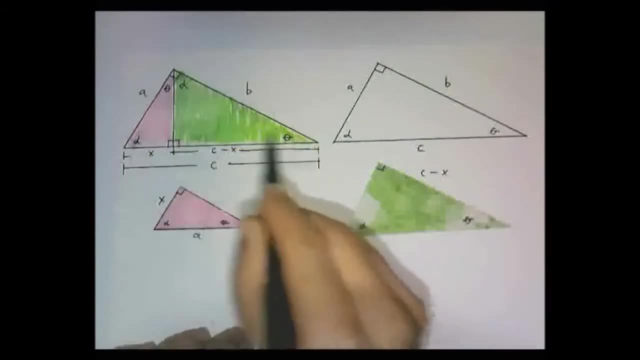 the angle alpha, See Angle alpha right here. And then side b, the hypotenuse of the green triangle is opposite the 90 degree angle. So opposite the 90 degree angle is this green triangle. This is the 90 degree angle. So 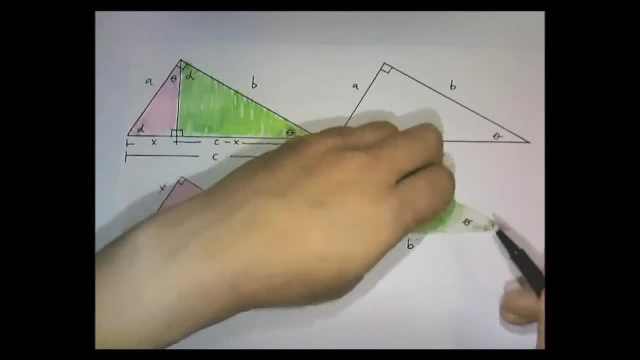 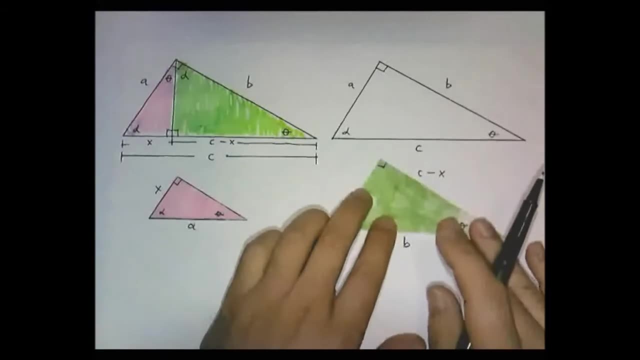 the hypotenuse of the green triangle is this: And the hypotenuse of this green triangle is: angle is side B right here. So side B is opposite the 90 degree angle here. side B is opposite the 90 degree angle there. Alright well, if you look at these, these two triangles, 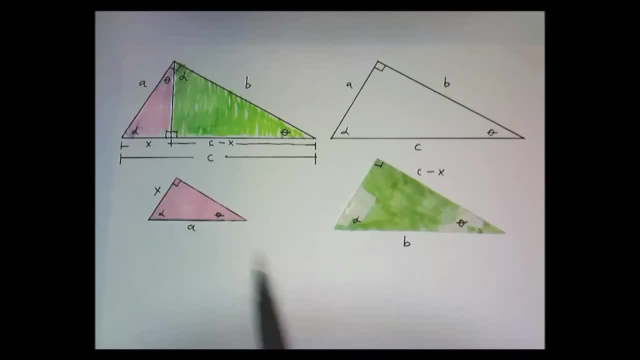 have the same shape- And they should, since they're similar triangles. they share at least two common angles. What that means is that the ratio of sides is proportional between all three of these triangles. So, for example, between these two triangles, the ratio of 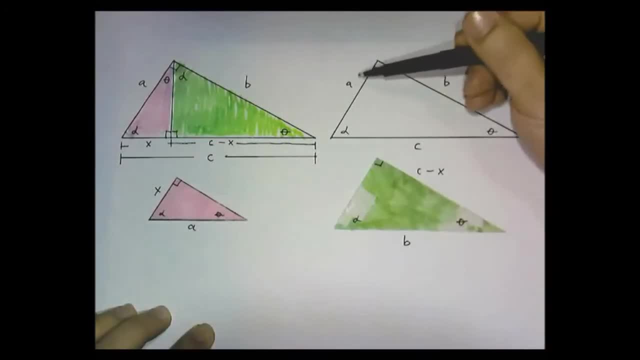 X to A is equal to the ratio of A to C. So let's write that The ratio of X to A, or X divided by A, is going to be equal to the ratio of A to C. Alright, and what we'll do. 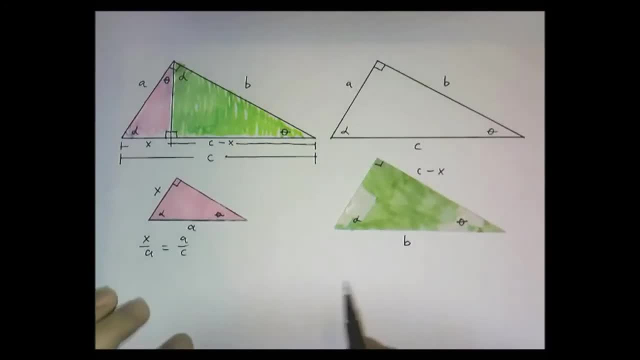 is: let's, uh, start to cross, multiply and start to simplify things here: X times C equals A times A or A squared Alright, and we're going to do the same thing, comparing these two triangles. The ratio of this side to this side, C minus X to B, is going to be equal to the ratio.